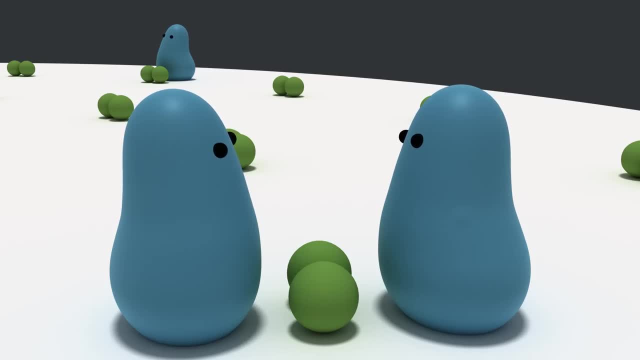 up. We'll start out by having only one possible strategy for creatures who run into each other. They'll just share, each taking a piece of food and going home, And because this strategy is so nice, we'll give it the name Dove. 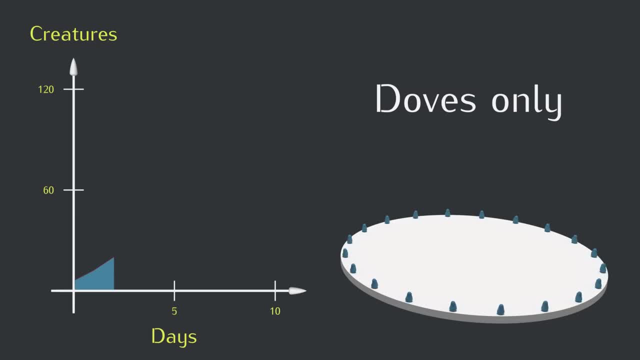 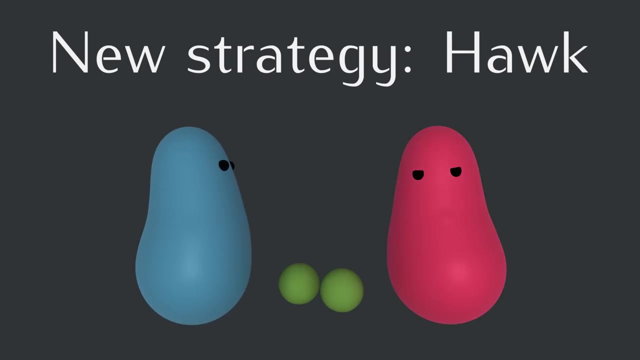 Alright, let's let things run for a bit. Alright, now let's add a new strategy called the hawk strategy. Hawks are more aggressive. If a hawk meets a dove, the hawk will go for the same piece of food as the dove eat half. 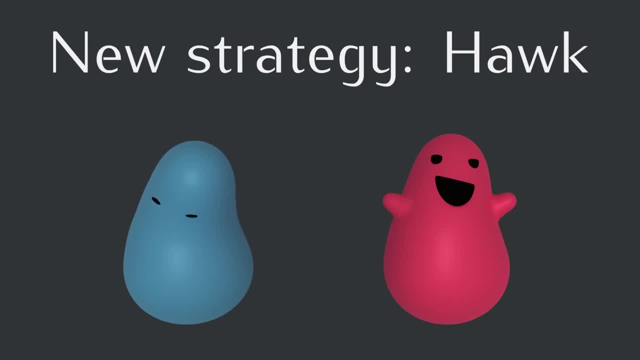 of it and then quickly eat the other piece of food, taking it for itself. This half food does complicate our survival and reproduction rules a little bit. So in this situation, a dove ends the day with half of food, so it'll have a 50% chance of surviving. 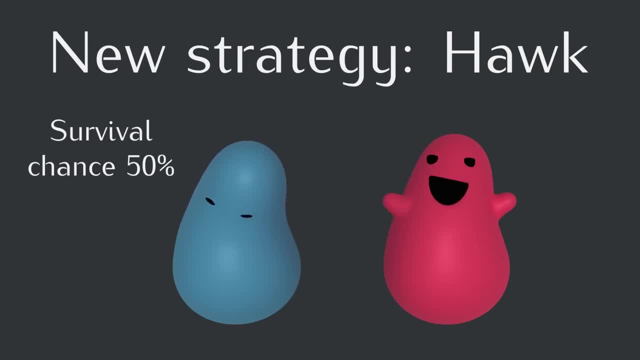 to the next day, and the hawk ends its day with one and a half food, so it'll survive for sure and also have a 50% chance of reproducing. Alright, now let's add a new strategy called the hawk strategy. Hawks are more aggressive. 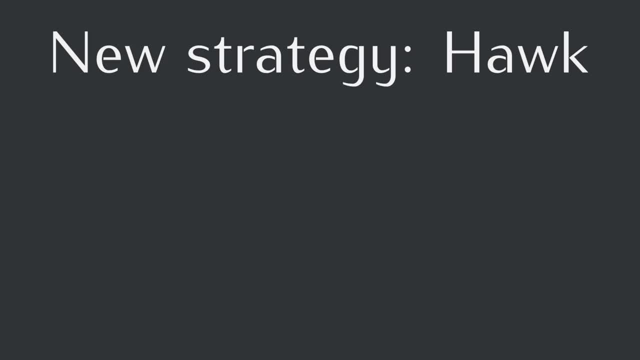 So it looks good to be a hawk, but it's also risky. If two hawks meet, they'll fight, And fighting is taxing. At the very least, they use a lot of energy and they might also get injured. So when hawks fight, each one gets a piece of food, but they spend so much. 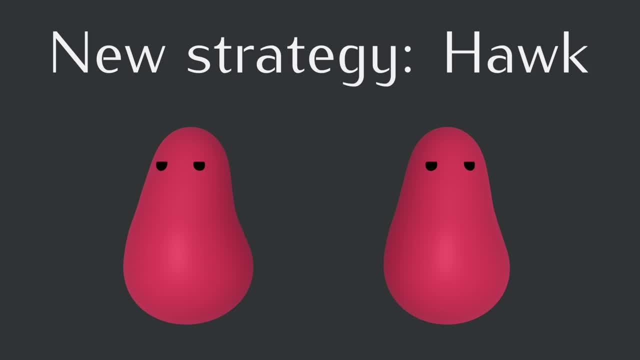 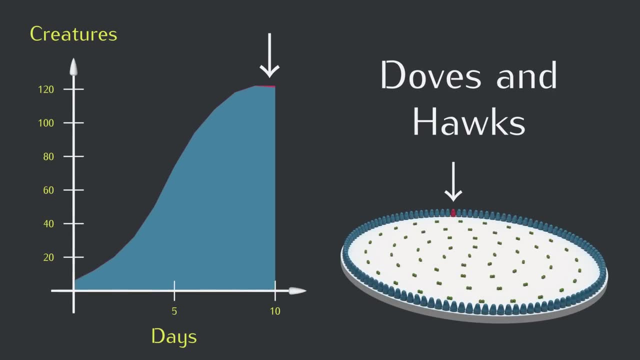 energy fighting that they use up all the benefit of the food right away and effectively go home with zero food, meaning they won't survive. So now let's try adding a hawk creature to our simulation and see what happens. Now is a good time to pause and predict what you think will happen. 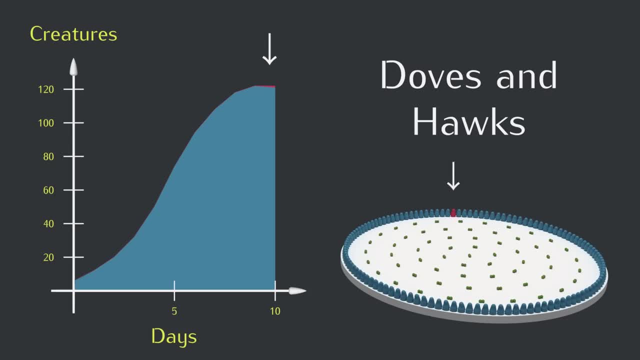 So that was an amazing Depth of Hope. If you enjoyed this video, I appreciate it so much. If you enjoyed the sequel, please leave a comment, and if you want to see more like this, I make sure to check out my other videos. 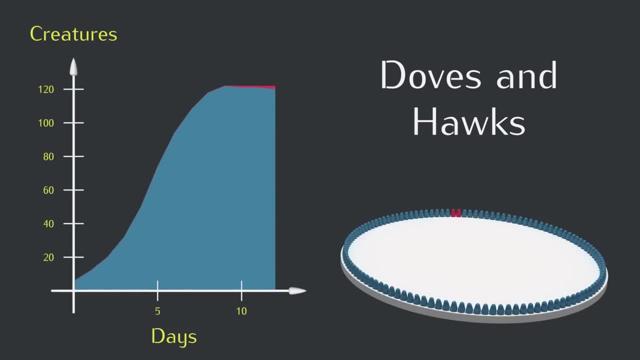 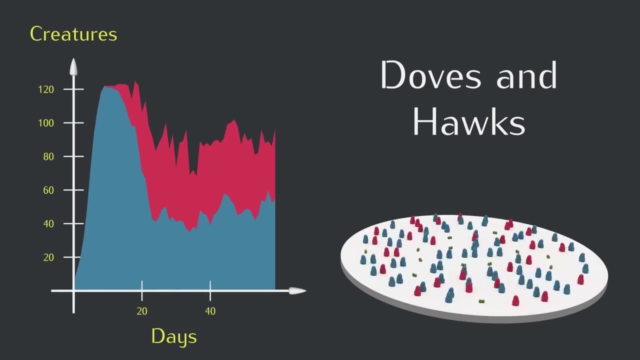 As always. thanks for watching and I'll see you next time. Alright, it looks like we have a mixture that fluctuates roughly around half and half, And there are also fewer creatures overall, even with the same amount of food. Here's an example of how natural selection doesn't necessarily act for the good of 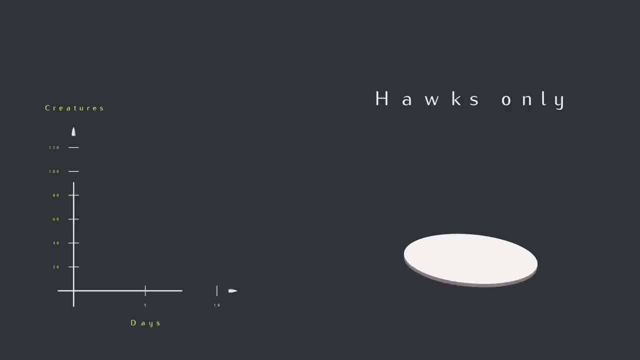 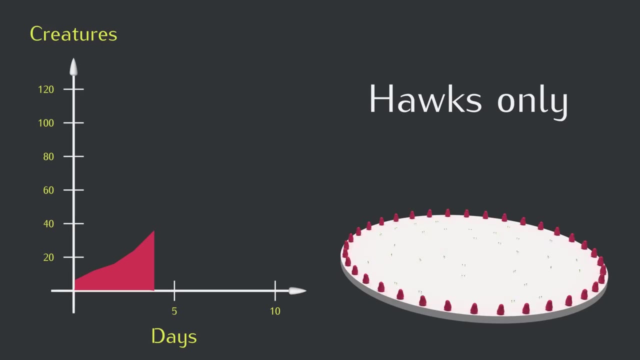 the species And to cover our bases. let's try starting with all hawks. Okay, not too surprisingly, they're tearing each other apart and their max population size didn't even reach half of the population size of the doves. Now, if we add a dove to the mix in the next day, what do you think will happen? 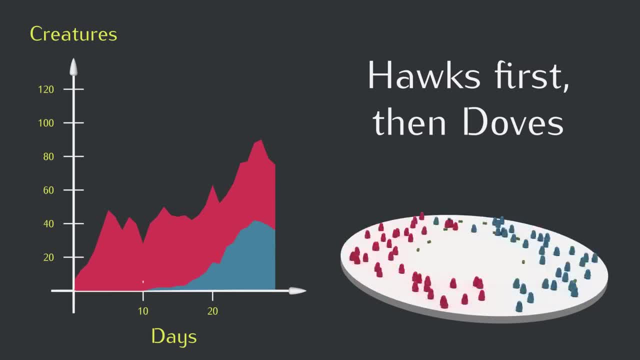 Okay, So it took the doves a little while to gain a foothold here, but eventually we end up in a similar situation with a fluctuating mixture of hawks and doves. So why do we care? Well, this is a situation where survival of the fittest doesn't help us understand what's. 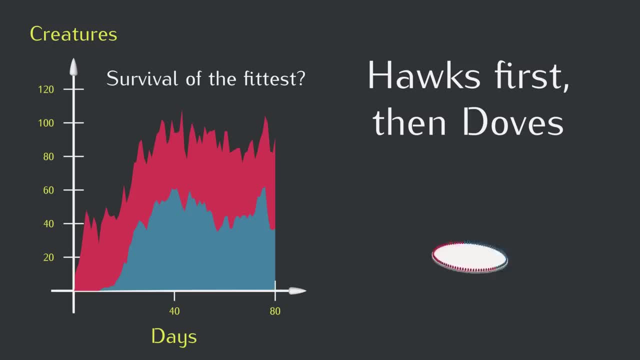 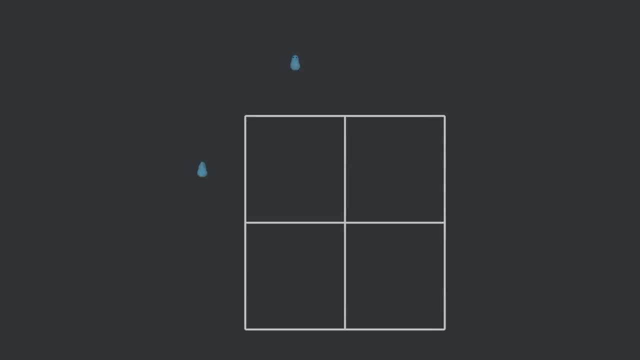 going on. There isn't one fittest strategy. We can get a better sense for why this is by translating our conflict rules from before into a table. If two doves face each other, they'll each get one food. If a dove faces a hawk, the dove gets half a food and the hawk gets one and a half. or 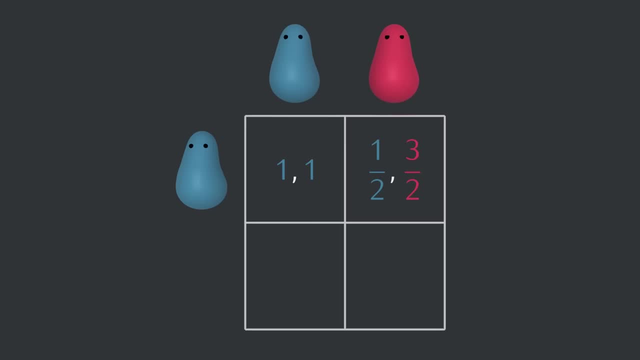 three halves food. And if we reverse perspectives, if a hawk faces a dove, they'll get half a food, They'll get three halves and one half, And when a hawk faces another hawk, they'll each end up with zero after they waste all. 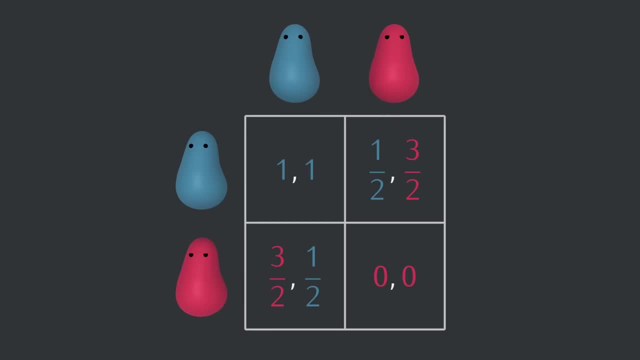 that energy fighting each other. Now that we have this table, let's imagine blobs that can choose which strategy they want to play. Say: I control the blob on top and you control the blob on the left. Say: you know that I'm going to play a hawk strategy, which of course I am. 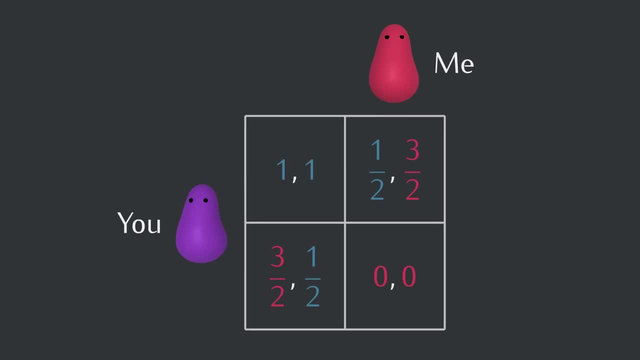 What should you do? Well, you're better off just backing down and taking your half food. That might be annoying, since it feels like I'm winning somehow, And you might be tempted to challenge me and also play hawk to teach me that I can't just. 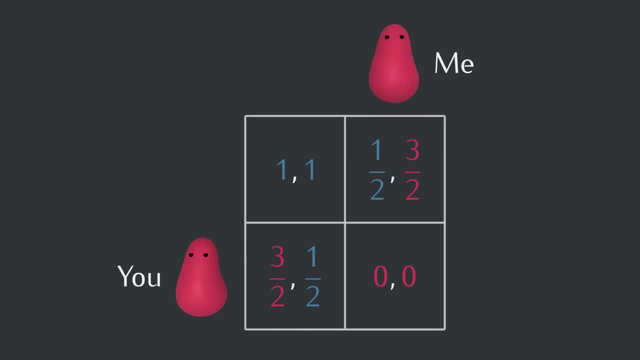 push you around. This could make sense if we were going to play this game against each other over and over again, as two humans might do, And that is something we'll talk about in future videos. But in this situation, we're just these simple blobs with no social structure interacting. 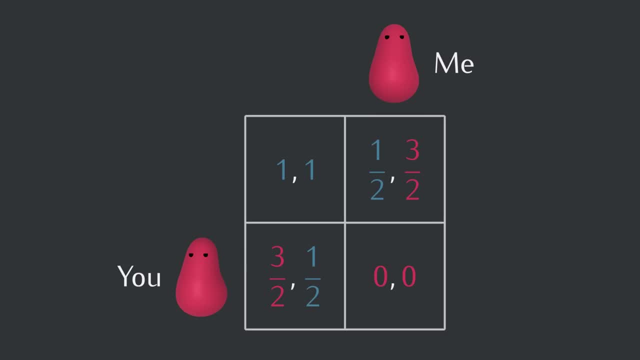 once, and even if we do see each other again, we won't remember it. So all that matters is how much food we take home right now, And if you want to maximize your chances of surviving and reproducing, you'll play dove. Discretion is the better part of valor here. 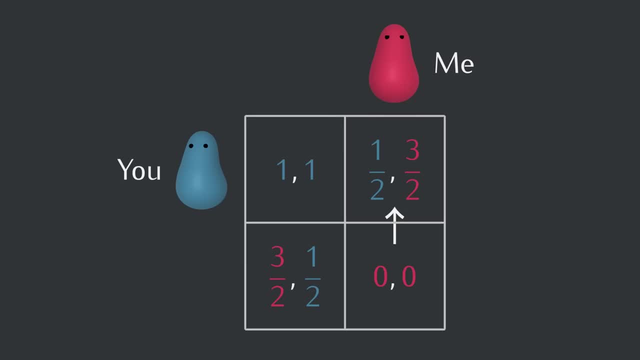 Let's record this by drawing an arrow. If we're in the right hand column because I'm playing hawk, the situation in the upper right square is the best you can do, Okay, in the other case, where I'm not so mean, you know that I'm going to play the. 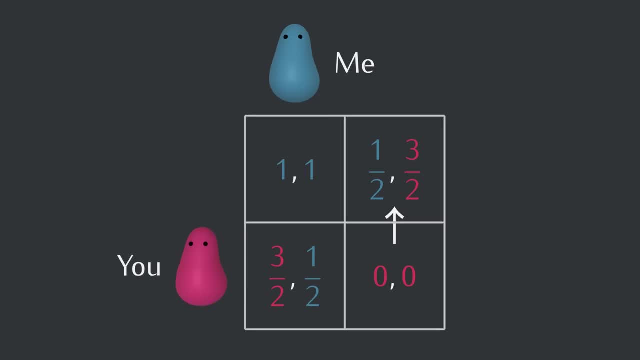 dove strategy. In this case you'll do better playing hawk. And here again, because you're a very smart human, you might be tempted to think about the future and want to reward me for playing nice and play dove yourself, but we're just. 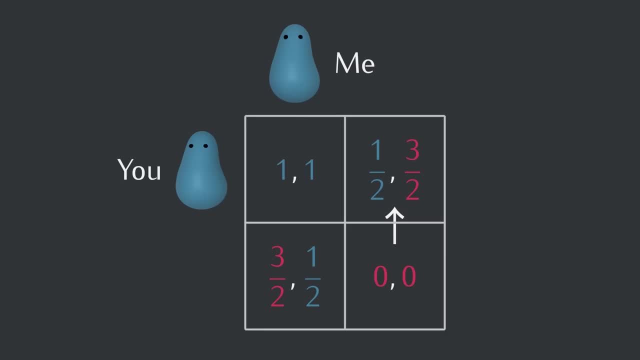 these really simple blob creatures who might never see each other again. So if you want to maximize your chance of reproducing, you'll play hawk And we can record this with another arrow. So now to complete this table, we can reverse perspectives and think about what I should. 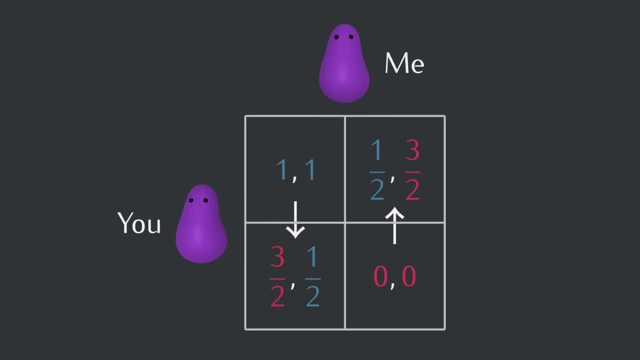 do in response to you, which I won't go through in detail. it's the same reasoning, but we'd get similar arrows in the rows here. These arrows all point to more advantageous strategies, And the interesting thing to notice is that there are two stable situations: either you 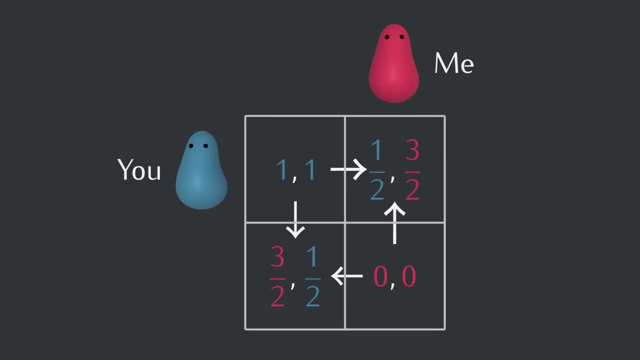 play hawk and I play dove, or you play dove and I play hawk. If we're in one of those two situations, we're going to have to play the dove strategy. And if we're in one of those two situations, we're going to have to play the dove strategy. 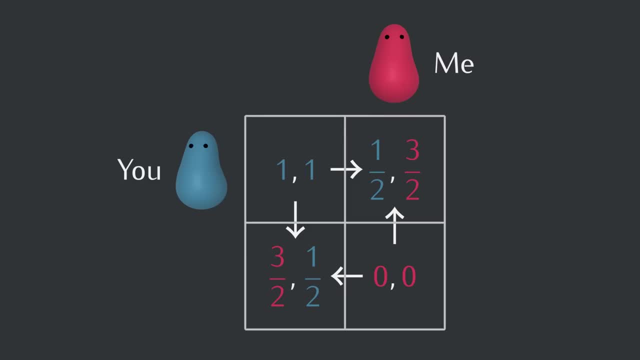 In those situations, either one of us would be worse off if we pick a different strategy. And, by the way, this way of analyzing choices is called game theory, which is a whole field of math, And a situation where nobody benefits from changing their strategy is called a Nash. 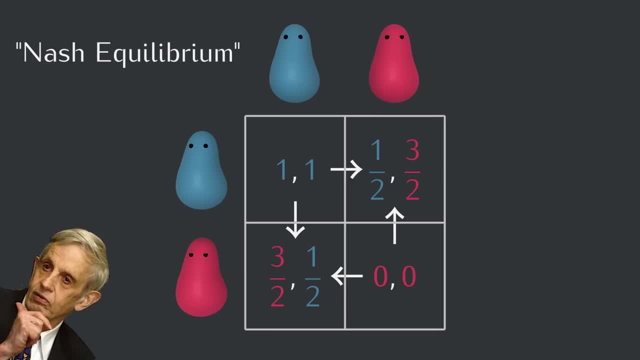 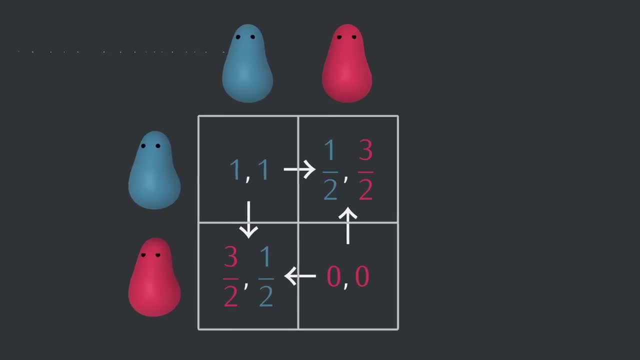 equilibrium named after John Nash, who some would say had a beautiful mind. So the best strategy isn't hawk or dove, it's to do the opposite of what your opponent is doing. When there are a lot of doves, it's better to be a hawk, and when there are a lot of 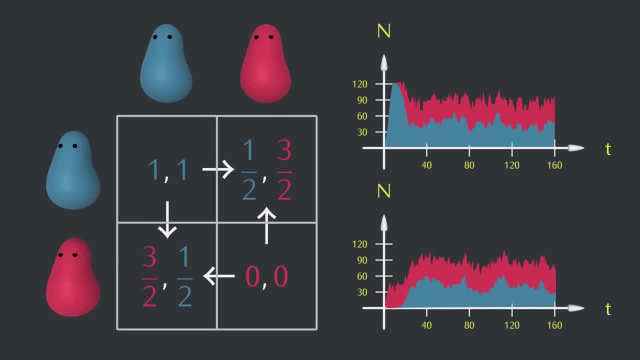 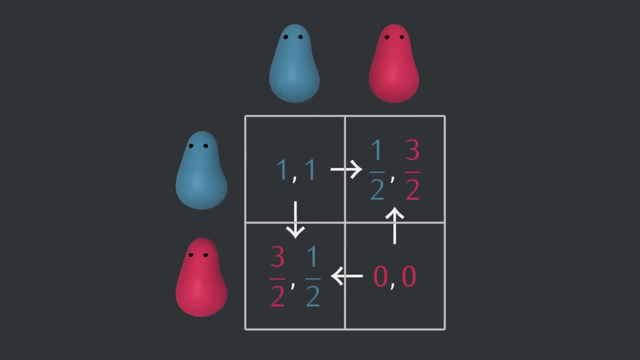 hawks, it's better to be a dove. There's some equilibrium fraction of doves that the population has always pulled toward Great. so we have the main conceptual point down, but we can deepen our understanding by calculating what that equilibrium fraction should be. 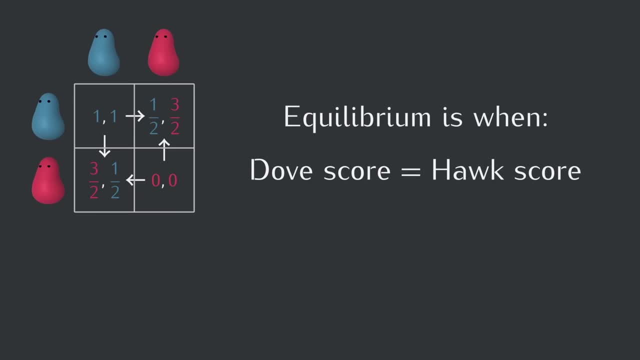 The population will be in equilibrium if doves and hawks have the same expected average score in a contest. Right Equilibrium is when, on average, we don't expect to change one way or the other, so we can't have one strategy doing better. 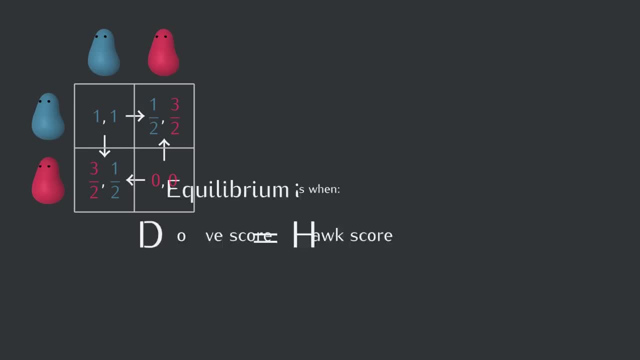 They're equal. Our goal is to find the fraction of doves that are equal to the average score in a contest, and that's what we're going to do. Let's first calculate the expected average score for a dove in a hypothetical example. 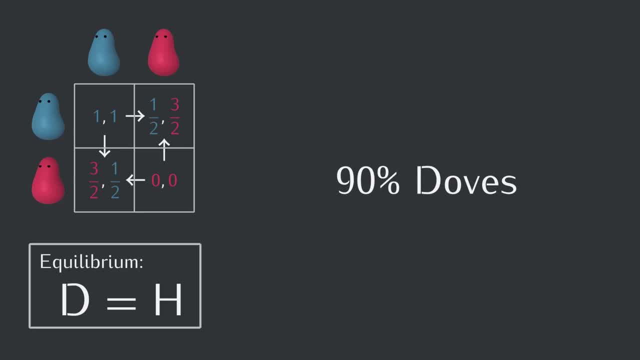 say where the rest of the population is 90% doves. So let's see, a dove will have a 90% chance of facing another dove, in which case it gets the dove vs dove payoff of one food, And a dove also has a 10% chance of facing a hawk. right, that's just the rest of the 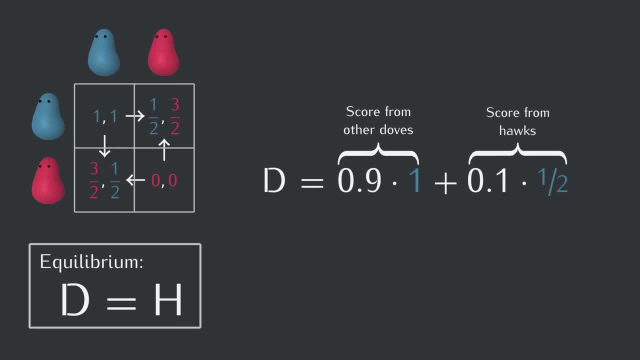 creatures, in which case it only gets a half of food. So overall, when a dove runs into another creature, when the rest of the population is 90% doves, it'll come away with 0.95 food on average. This number is pretty meaningless on its own, but once we calculate the expected hawk score. 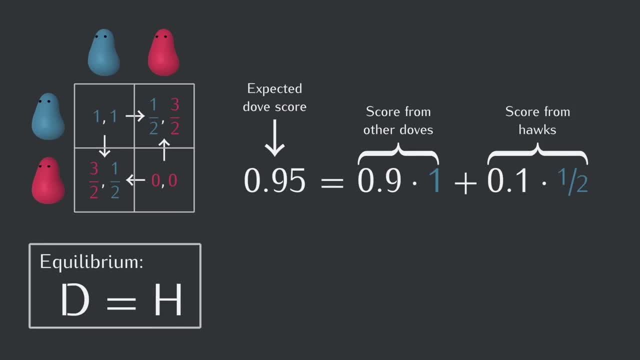 we can compare the two to see whether the equilibrium condition is met. So let's do that. let's find the expected hawk score. It could be good to pause and try to do this yourself, to make sure it all makes sense, maybe even rewinding to watch the dove part again. 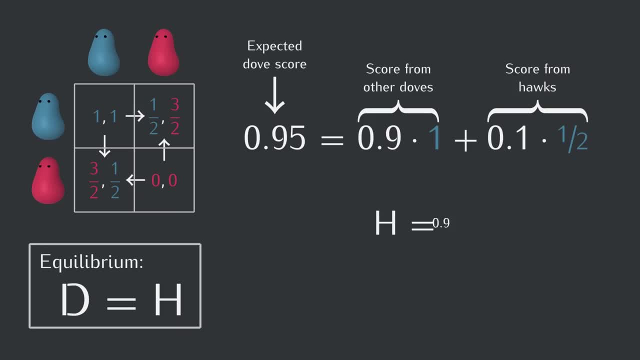 Okay, Just like before. So the population is 90% doves, and against a dove. a hawk gets one and a half or three halves pieces of food And again, there's a 10% chance of running into another hawk, in which case our hawk. 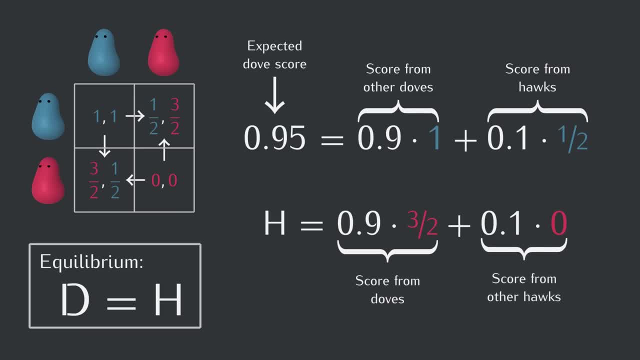 goes home with 0 food and this comes out to 1.35 food on average. Now notice that 1.35 is more than 0.95, so at 90%, doves, hawks will do better and we'd. 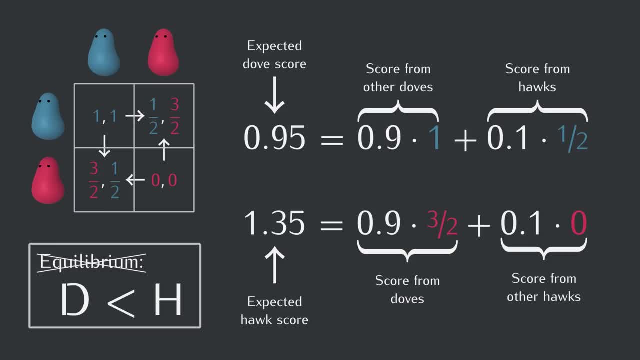 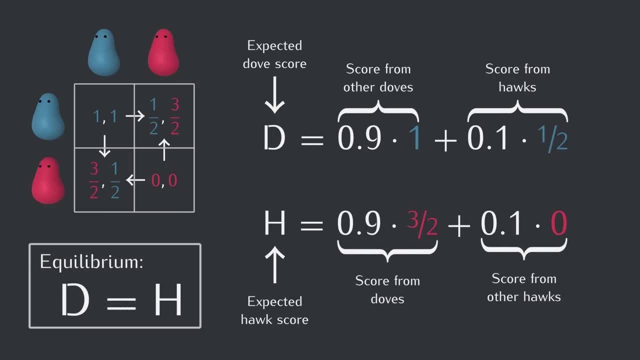 expect the fraction of hawks to increase in the next generation. So it's not equilibrium, Not 90%. Now to find out what fraction of doves does meet the equilibrium condition, we can write the fractions of doves and hawks as variables, instead of just guessing at specific numbers. 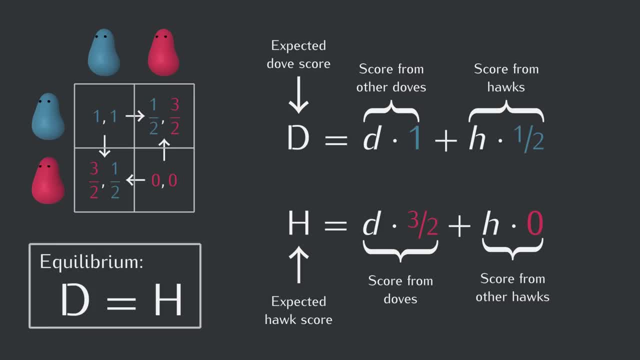 And you might be saying right now: wow, that's a lot of letters, which is a fair point, but we're almost there and our next step is actually to get rid of one of those letters, so there's a nice treat already. 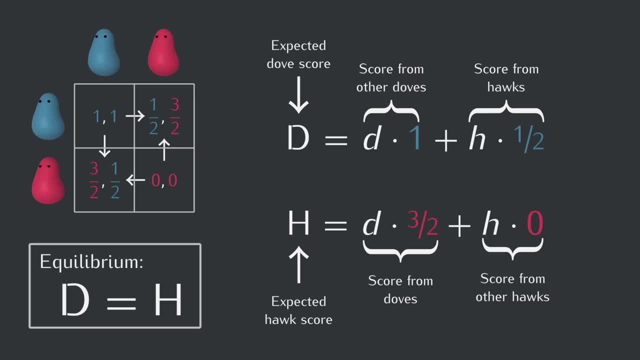 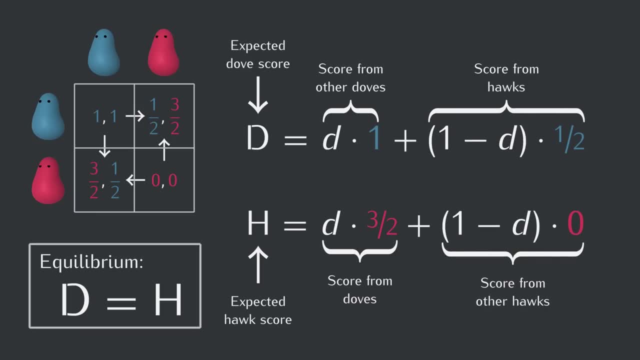 Doves and hawks make up all the creatures, so their fractions have to add up to one, And this means we can replace the small h with 1 minus small d, And now the n-th is equal to 1 minus d. And now the expected dove and hawk scores are both written as functions of one variable. 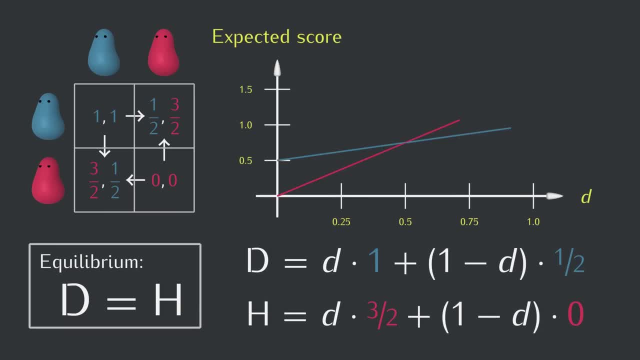 and the same variable, so we can graph them on top of each other. The expected scores are equal when the graphed lines cross and indeed the equilibrium condition is met at 50% doves. And if we run a simulation with way more creatures than before- unfortunately too many to animate. 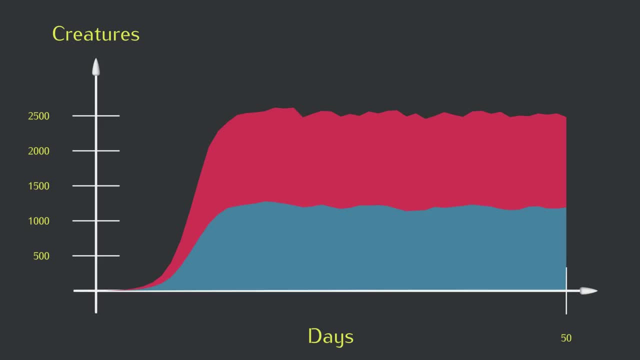 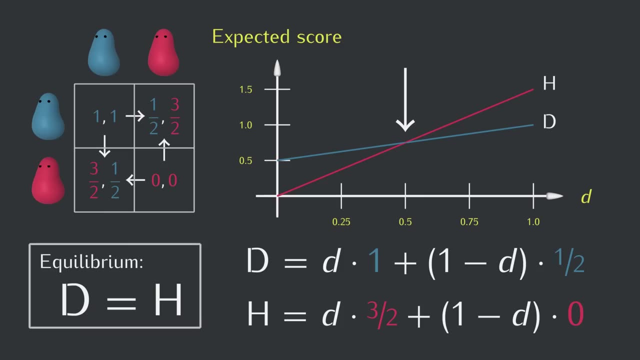 the randomness smooths out a bit and we can see that the prediction is true. Okay, so it might feel like that was kind of a lot of work just to verify, but it's not. The fraction of doves isn't always going to be one half. 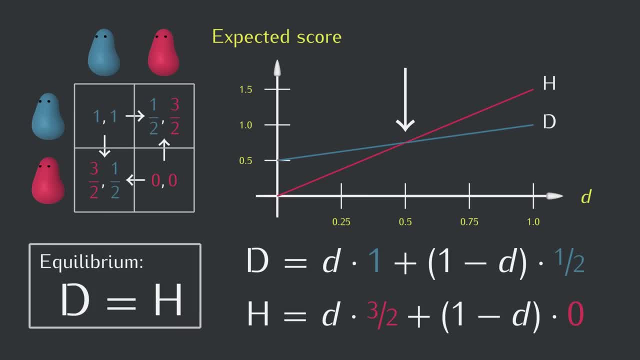 It depends on the numbers in our payoff grid. The most interesting number to play with here is the hawk versus hawk payoff. So far we've been saying that the hawks each get one piece of food but waste all the energy of the food on fighting. 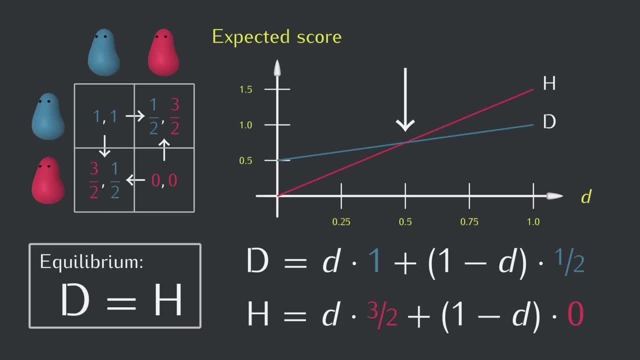 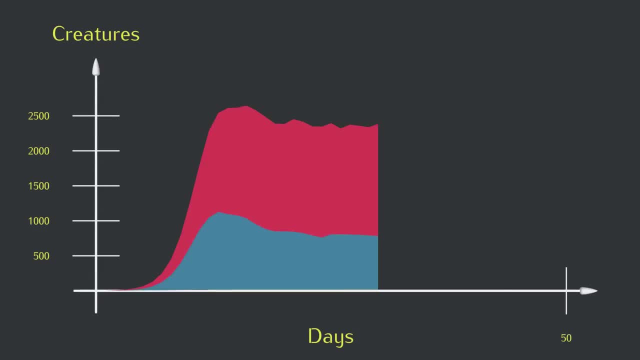 But what if, instead, they only waste most of the energy, not all of it, and go home with a score of one fourth. Plugging that in, we see the population move toward one third doves, And again we can see this borne out in the simulation. 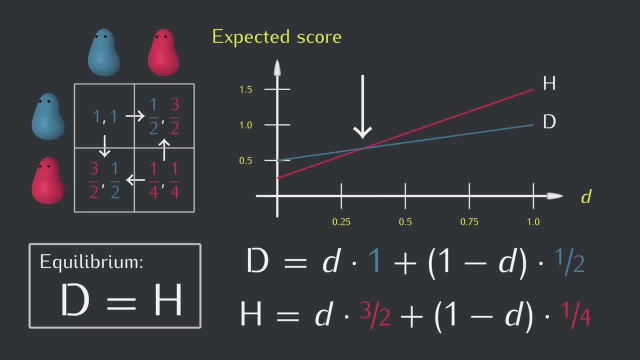 At this point, congratulations. We have a pretty detailed understanding of how populations of hawks and doves work And, as basic as this model is, with only two simple strategies, it's a powerful starting point for analyzing behavior in the real world. 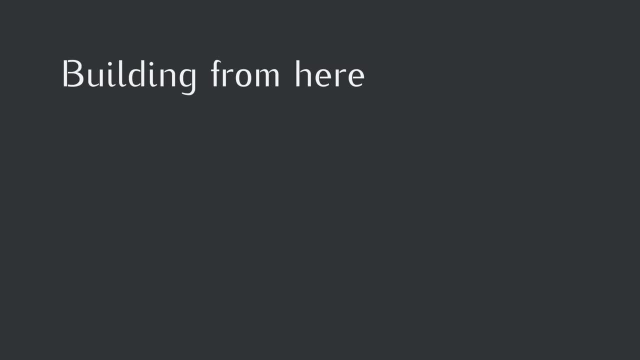 And before we go, I want to give you some teasers for how we'll build on this to get closer to reality in future videos. First, creatures in the real world can play more than one strategy. So instead of having their behavior completely determined by a single gene, our creatures